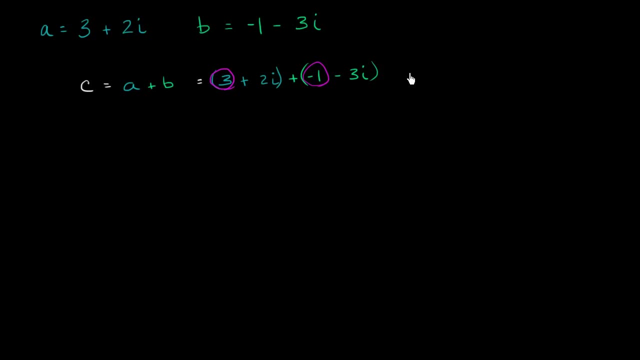 So I could add the 3 to the negative 1 to get 3 plus negative 1 is 2.. So I get a real part now of 2.. And then I can add the two imaginary parts. So if I have 2i minus 3i, that's going to be negative 1i. 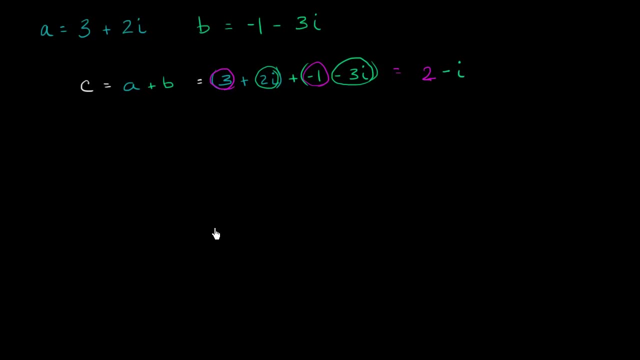 Or I could say that's going to be negative i. So, just like that, I added the two real parts, added the two imaginary parts and I got 2 minus i. And we could also visualize this on the complex plane. We could do that using an Argand diagram. 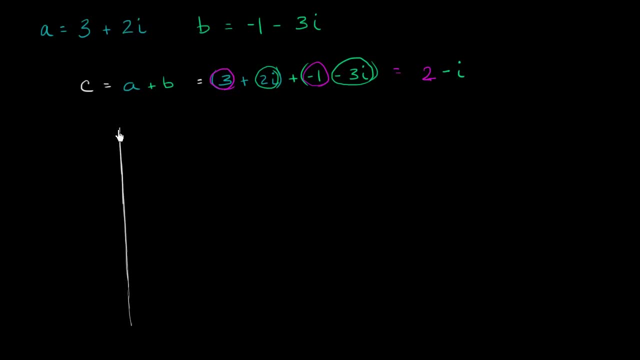 In an Argand diagram. we represent each of these complex numbers as vectors on the complex plane. So that's our imaginary axis, This is our real axis, And a is 3 plus 2i. So 1,, 2,, 3 along the real axis. 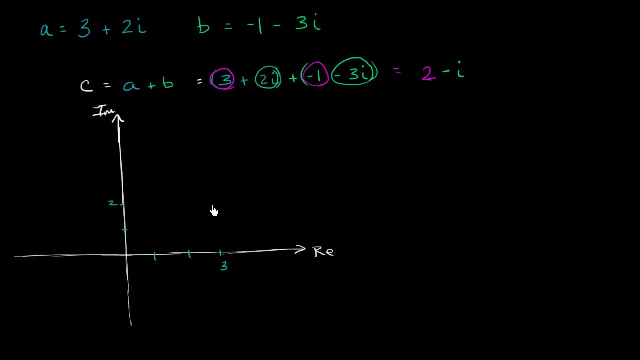 And then 2 along the imaginary axis. The imaginary part is 2. 2i. So 3 plus 2i gets us right over there, And I'm going to represent that as a vector, As a vector where its tail is at the origin and its head is at the coordinates. 3 on the real axis. 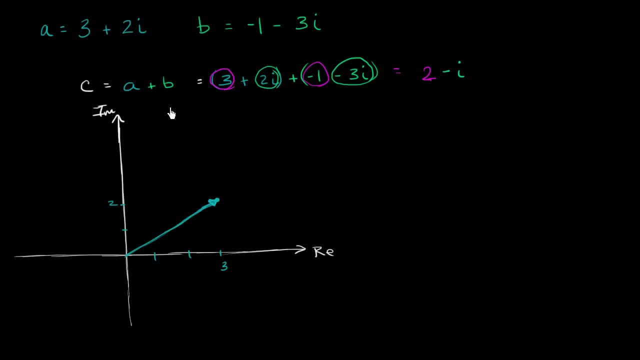 2 on the imaginary axis. So that right there on my Argand diagram, is my representation of vector a. Now let's do the same thing for vector b. It is negative: 1 along the real axis, 2 along the imaginary axis. 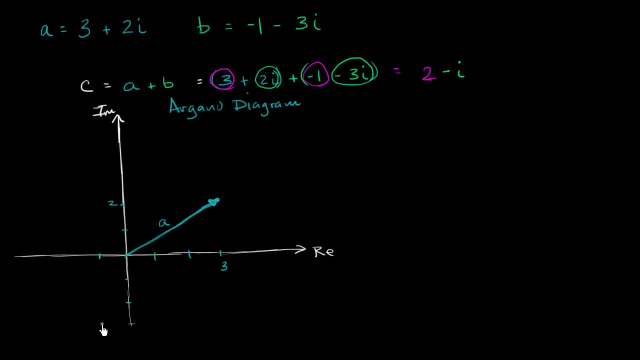 1,, 2,, 3.. So it sticks us right over there If we represent it as a vector. vector or complex number b could be visualized this way, And now, when we add a plus b, you could add them the exact same way that you would add vectors. 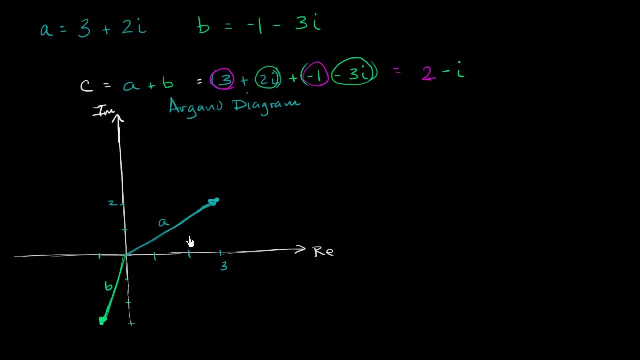 You take the tail of b or you can essentially shift b over. So you take the tail of b and you put it at the head of a, But it's the same thing. So when you go down 3 and you go to the left, 1.. 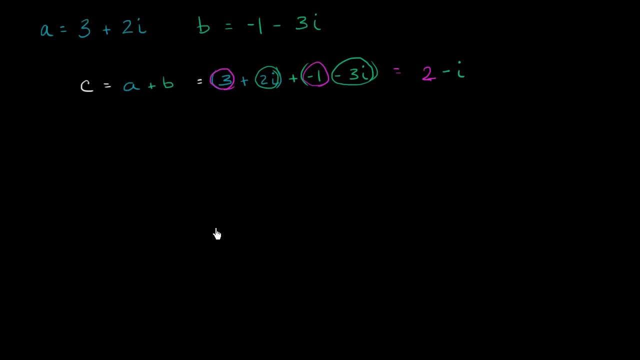 Or I could say that's going to be negative i. So, just like that, I added the two real parts, added the two imaginary parts and I got 2 minus i. And we could also visualize this on the complex plane. We could do that using an Argand diagram. 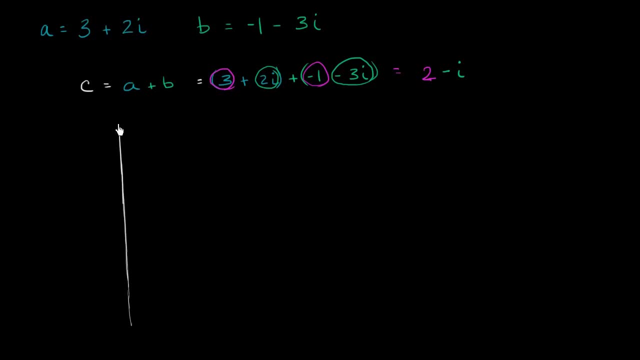 In an Argand diagram. we represent each of these complex numbers as vectors on the complex plane. So that's our imaginary axis, This is our real axis. This is our real axis, And a is 3 plus 2i. So 1,, 2,, 3 along the real axis and then 2 along the imaginary axis. 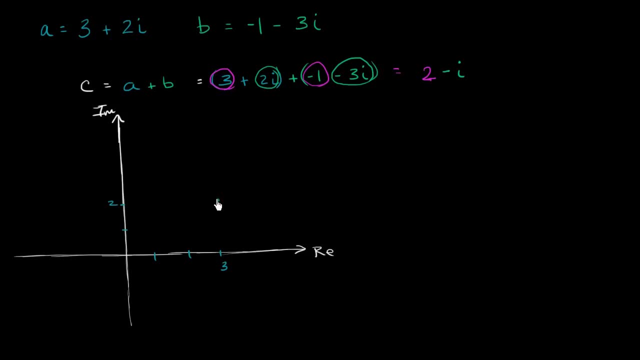 The imaginary part is 2. 2i. So 3 plus 2i gets us right over there, And I'm going to represent that as a vector, as a vector where its tail is at the origin and its head is at the coordinates. 3 on the real axis, 2 on the imaginary axis. 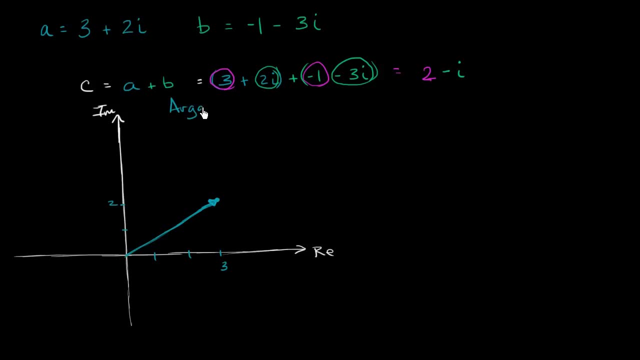 So that right there on my Argand diagram is my representation of vector a. Now let's do the same thing for vector b. It is negative 1 along the real axis and negative 3 along the imaginary axis: 1,, 2,, 3.. 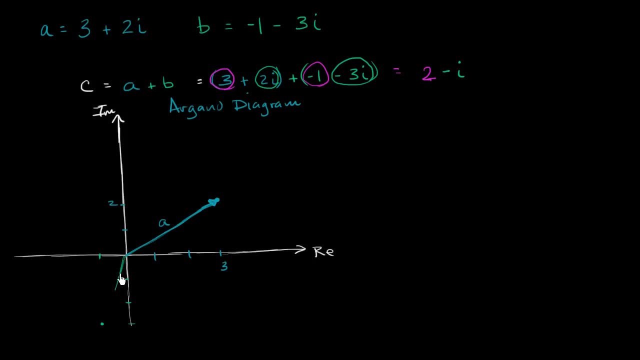 So it sticks us right over there If we draw, if we represent it as a vector, vector or complex number b could be visualized this way, And now, when we add a plus b, you could add them the exact same way that you would add vectors. 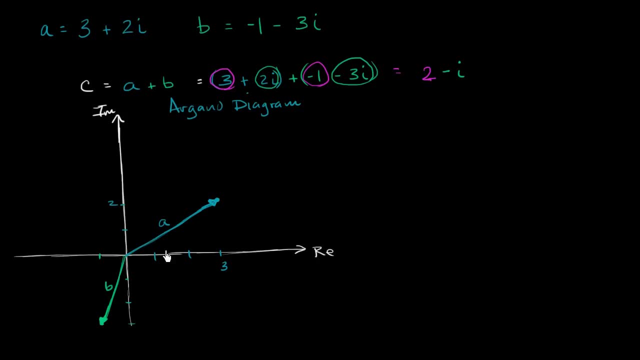 You take the tail of b or you can essentially shift b over. So you take the tail of b and you put it at the head of a, But it's the same thing. So you go down 3 and you go to the left 1.. 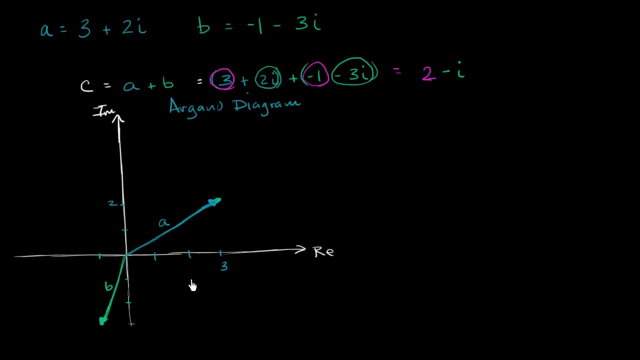 So you go down 3 and you go to the left 1.. So it's going to put you right over here. So all I've done is I've shifted b over to this part so that its tail is at the head of a. 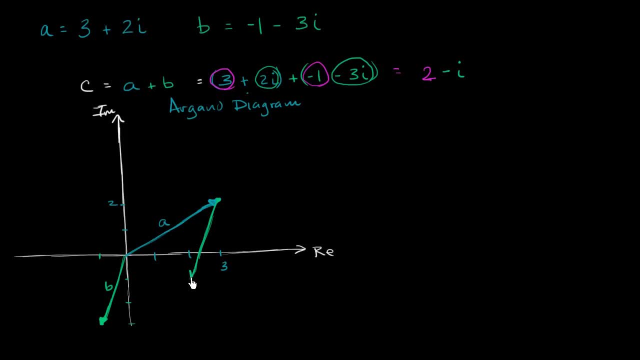 So it goes right over there. So this is vector b or not vector. this is complex number b. So this is b right over here. And notice now, if we start at the tail of a and we go to the head of this shifted b.